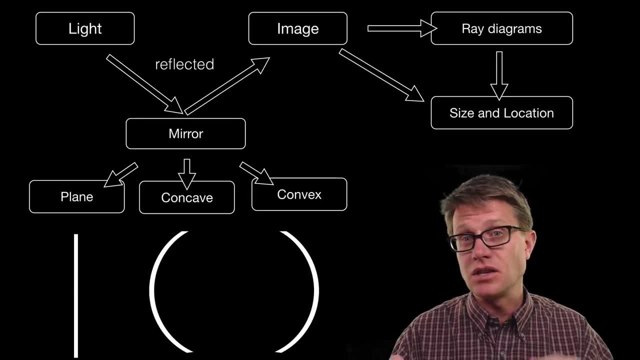 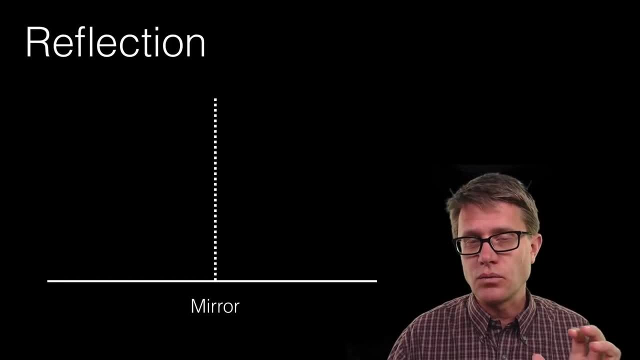 rays go And therefore we can figure out: where is that image? Is it a real image or a virtual image? We will talk about that in a second- And how big is that image actually going to be? And so let's remember, reflection is. 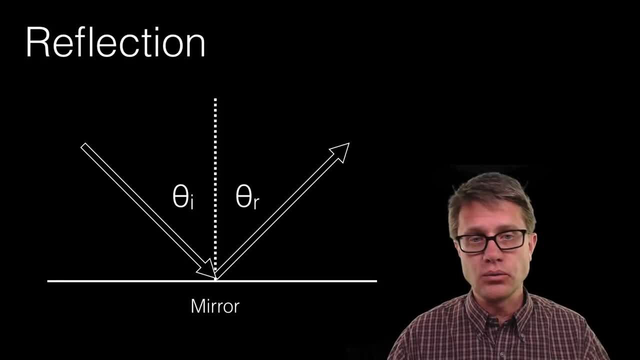 going to be light bouncing off a surface, And our only rule is that the angle of incidence- the angle between normal and the way at which the ray comes in- is equal to the angle of reflection, And so I took this picture of myself using a Bozeman Science shirt And 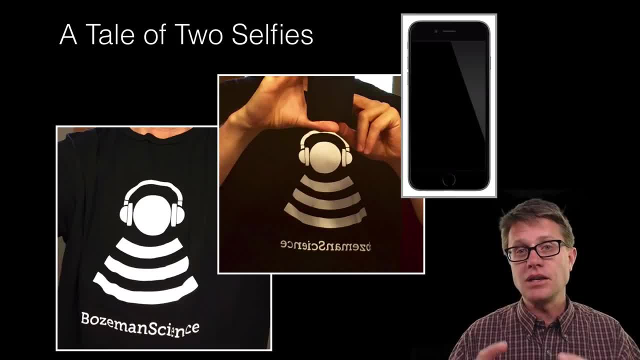 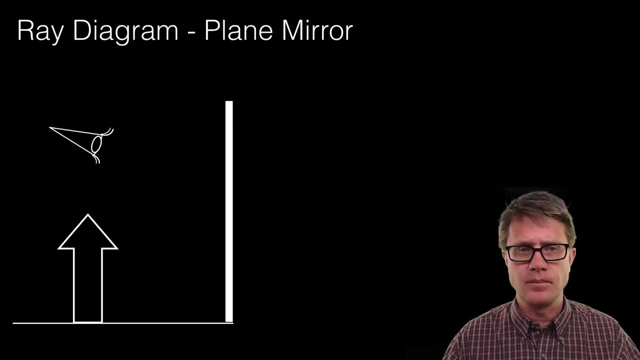 I took it with my phone, using both the front facing and rear facing camera, And in the rear facing camera I stood up to a mirror. Can you figure out which of these images was taken using a mirror and which was not? Well, probably. And so let's get to why they look a little bit different. And so to draw 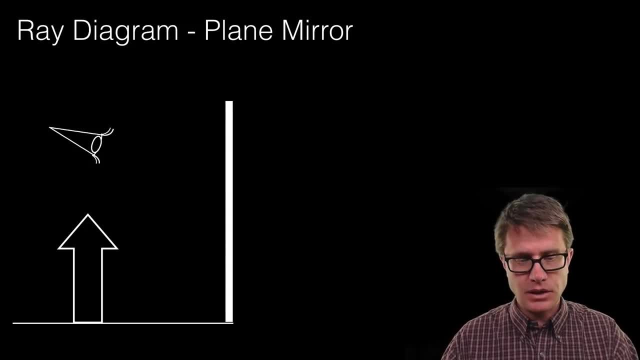 a ray diagram for a plane mirror. it is fairly simple. So let's say: this is our eye, This is the object, It is just an arrow pointed up And we want to draw how that mirror creates that image. Well, the first thing you have to realize is that there is going to be a 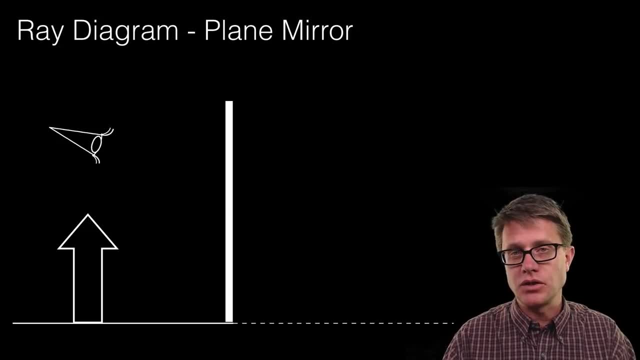 virtual side to the mirror, And so every time in a ray diagram you see dotted lines that they are not real, They are virtual. In other words, you are facing a mirror and there is no area back here, It is just created in your mind. You could not go visit it. It is a virtual. 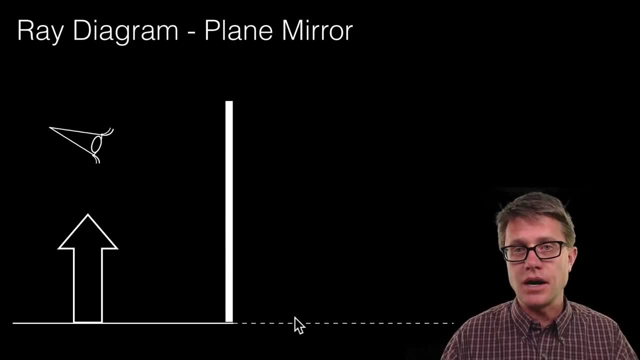 area. And so the first thing you do with a plane mirror is you draw the object in an equal distance away from the plane mirror. So I have drawn a virtual image. It is the same exact size, It is upright in nature, And now we are just going to draw in the ray. 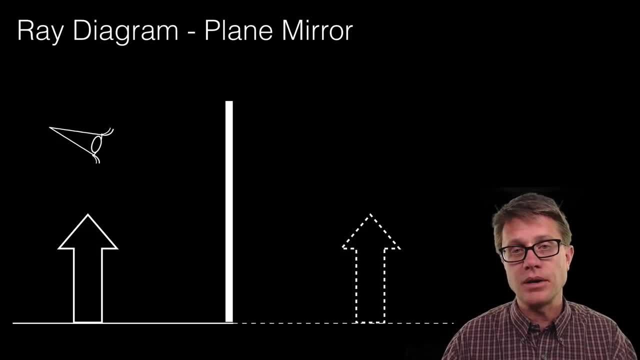 diagram. And so what you do is you choose a point on the top of the object And you just draw a straight line to the eye. Now, it is dotted on this side because this is virtual, remember, and it is going to be a straight line to my eye. We know the light. 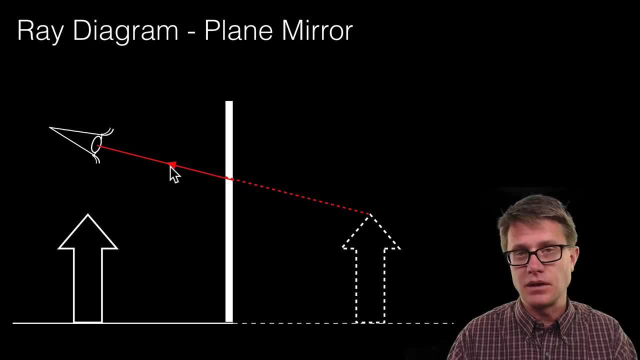 is going into my eye. We are not shooting light out of my eye. That is why the arrow is in this direction. Once I have done that, now I take that same real object and I am going to draw a line like that. You can see, the angle of incidence equals the angle of. 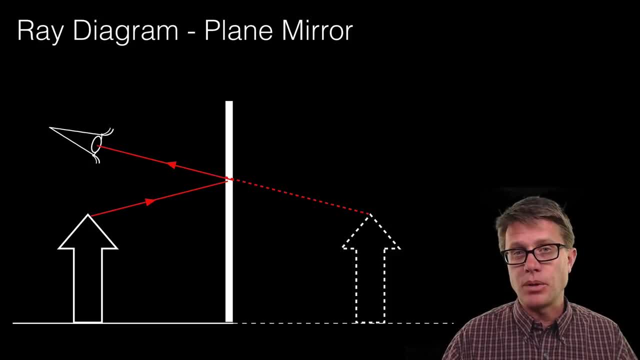 reflection and it goes right back to my eye. like that: Now we choose a part of the object, let's choose the bottom part of the object, and we do the same thing, Draw a line to my eye, virtual to real, And now I am going to draw that in the real world. like that, And 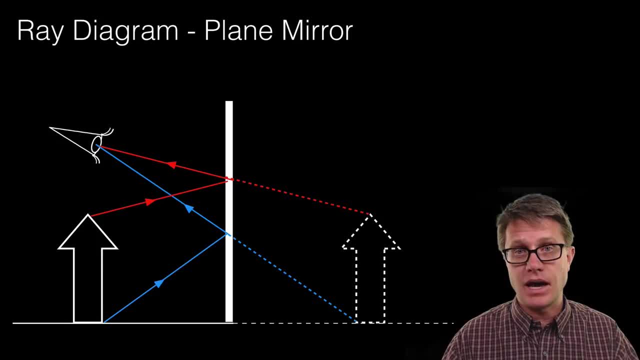 now I have got my ray diagram for my plain mirror. It is as simple as that. Again, draw the virtual image on the other side And then connect the dots And then make sure that you have got. angle incidence equals the angle of reflection, And so why does it look weird? 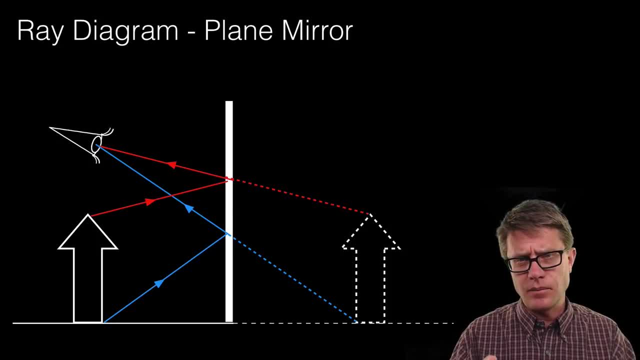 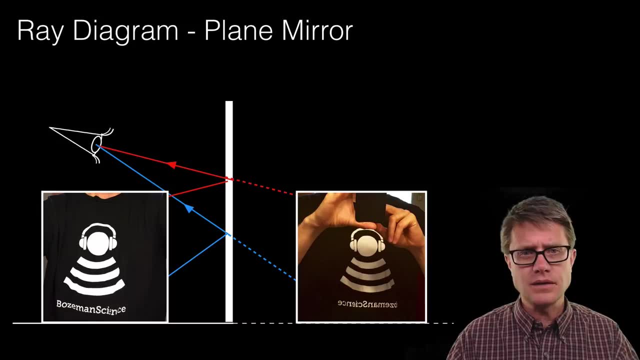 in a mirror, And what I mean by weird is you notice that my shirt was backwards, And so with one of those selfies it looked like that, And on the other one it was reversed. So why is that, Well, what we are doing? I could turn it around, it would look normal, is that the? 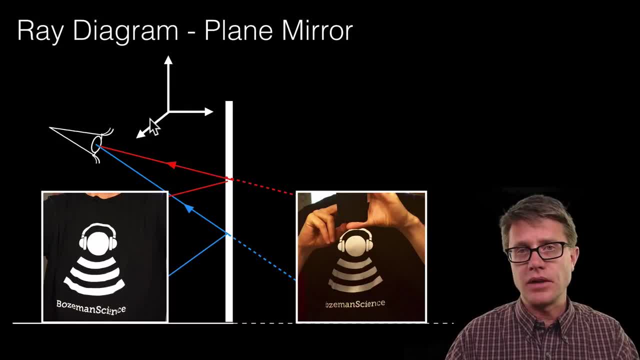 up down right, left, is not being reflected. What is really being reflected is the plain into the mirror, And so we get reflection of that. And so, as your shirt, as you are wearing the shirt, you are really wearing it not facing you, but away from you, And that away from. 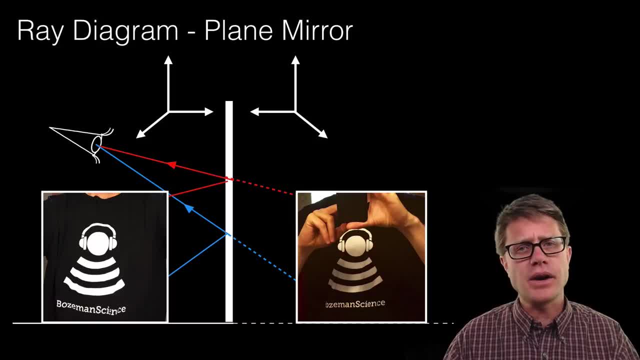 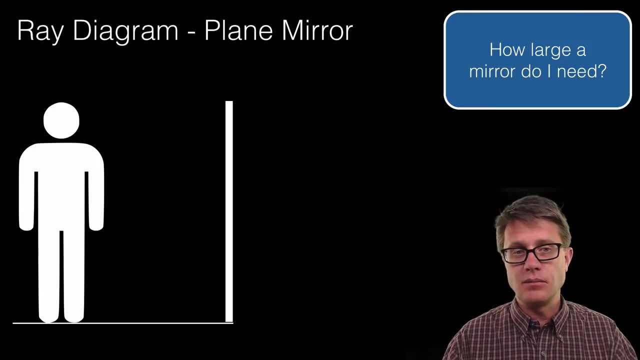 you image is great. It is going to be what is reflected, And so let's practice this. Imagine you are standing next to a mirror and I ask you the following question: How large a mirror do I need to see my whole image using a plain mirror? And so, to practice, I would encourage you to pause. 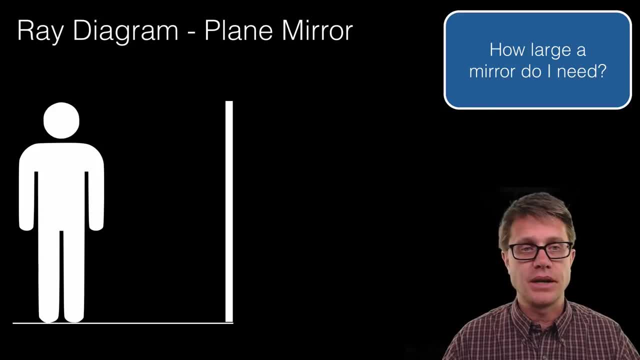 the video and draw this one out, But I am going to do it for you right now, And so the first thing you do is you create the virtual version of yourself on that side. You then start at the top, And so I am going to draw an arrow to my eyes. How did it get there? 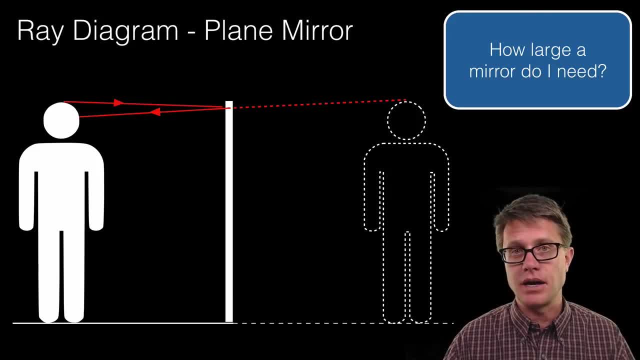 It went from the surface of my head, bounced off and came back to my eye. Now I go to the bottom of the image, It goes to my eye And then I bounce it off like that. And so if you make sure that it is going in, 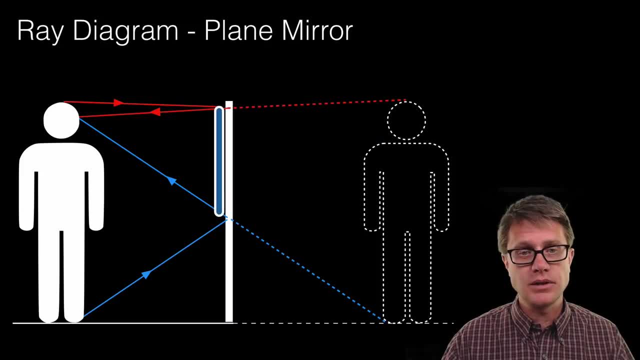 the right direction. how big is the mirror going to be? It is really small. It is actually going to be half of my height And I can still see my feet in the mirror because it is going to be reflected like that. Now let's move on to a concave mirror. So a concave, remember. 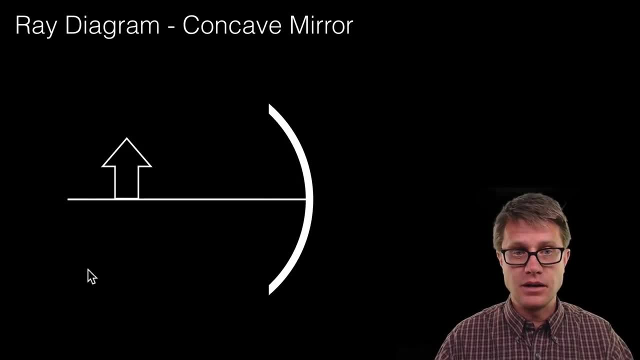 we are going into a cave like this, And the object is over here, And then the observer. the observer is somewhere out here, So you are looking at the image, And so for this one we have to define a couple of points. First, we have got the center of curvature. 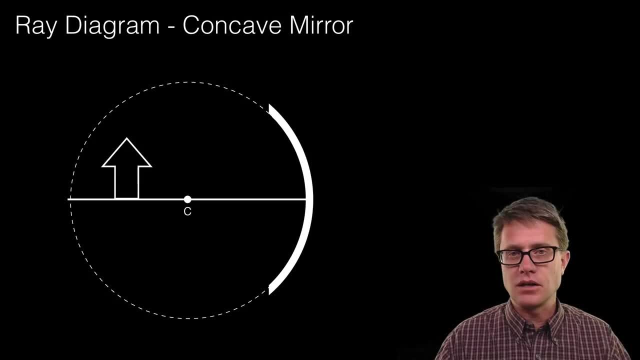 or the center of that mirror. So imagine that as a center, So the radius to the mirror goes right back to that center point. We are also going to add a focal point, So the focal point will become important in just a second. But when you are drawing a ray diagram for a concave, 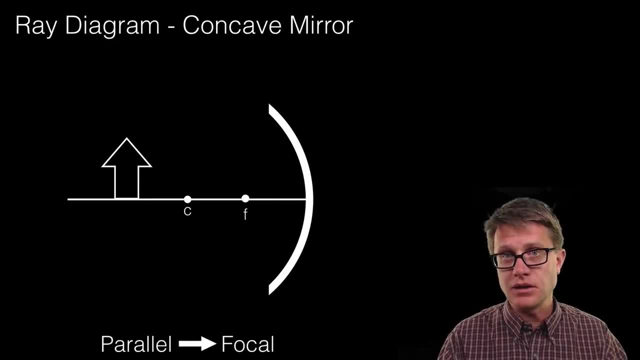 mirror. what you will do is always start with a ray that is parallel to the mirror, Then go through the focal point, Then you are going to draw the center of the mirror And then you go through the focal point And then go back to parallel. So let me show you what. 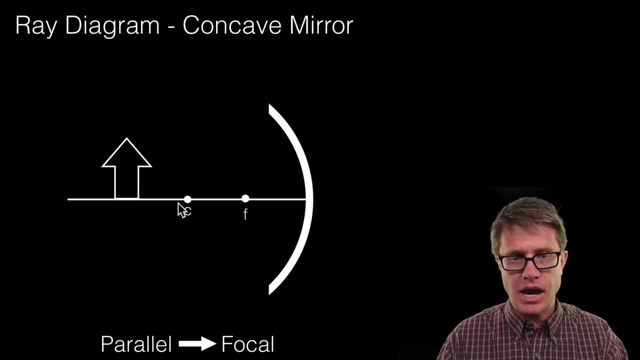 that looks like. So you need to know where the focal point is. Also, it is going to be half of the center of curvature Or you will see sometimes this written as F and this as 2F out here. But again, we are on this side of the image over here. First thing you do: 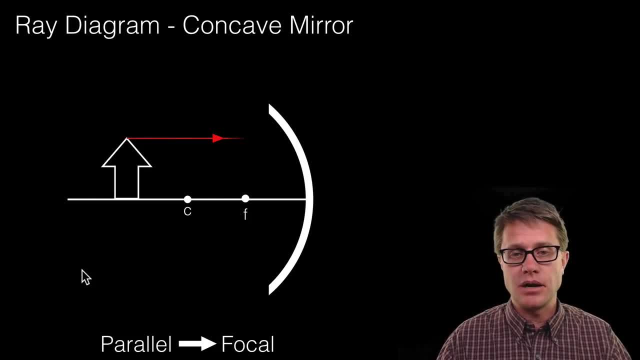 is, you draw a ray now from the real object And it is going to be parallel to the mirror, And then that ray is going to go through the focal, And so that is what is neat about the focal length and the focal point, Because if it is ever parallel to the mirror it is going to bounce off. You can see the 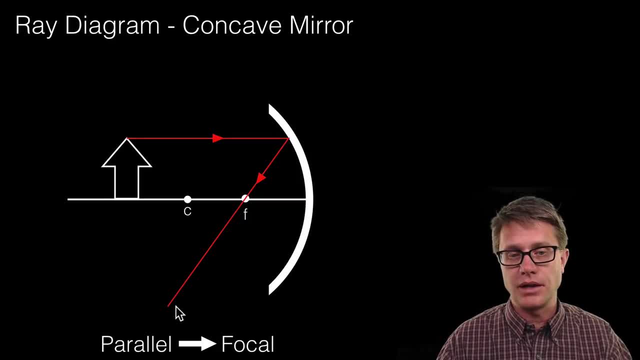 angle of incidence equals the angle of reflection And it goes right through the focal point like that. So first go parallel through focal And now we are going to take that same top of the image and we are going to go turn it around. So now we are going to draw through. 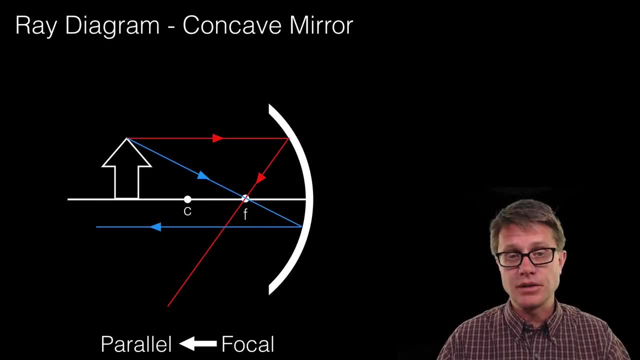 the focal, And then that is going to create a parallel. So it is the opposite of that rule. So now we look at where is the light coming? So here it is coming out, Here it is coming out, And so where is our image going to be? Well, it is going to be right here. 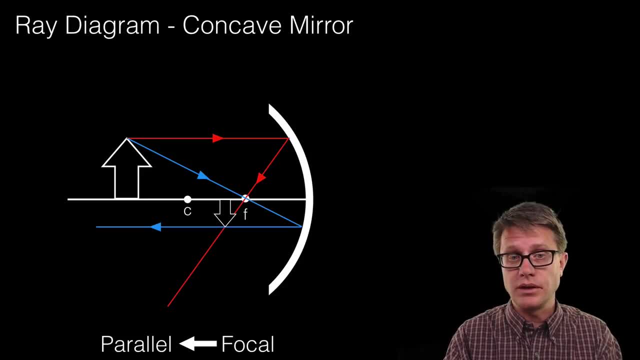 not a dotted line. It is a real, true image right there. So it is a real image. You can see it is smaller in size and it is going to be inverted, So it is going to be upside down. Now, a real image. you could take a piece of paper, put it there and you would actually 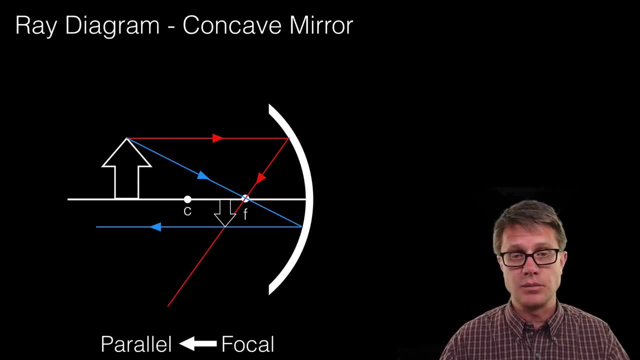 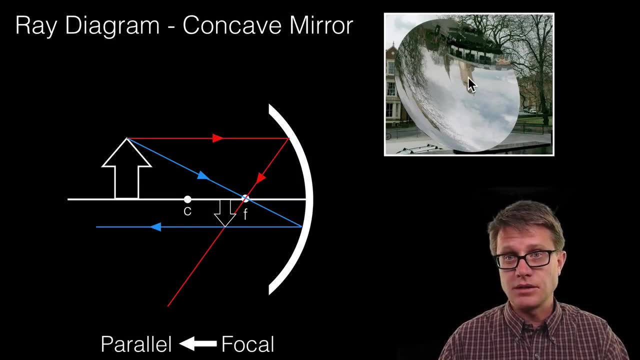 see the image on the paper itself. It is not a virtual image at all. If you look at this, here is a concave mirror, So the camera man is taking a picture of it and you can see the buildings behind him are inverted upside down and they are much smaller in size And 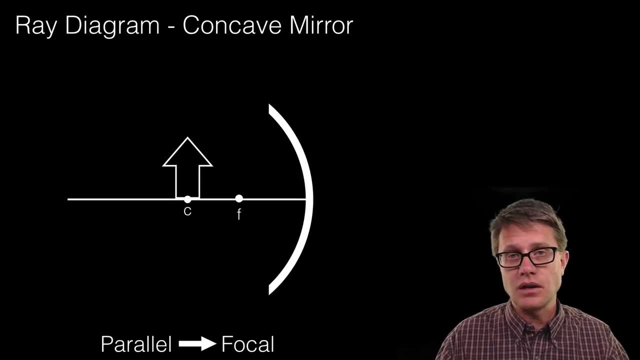 that is going to be a concave mirror. Now I have moved the object up here to the center of curvature. I would encourage you again. pause the video and try to draw this one out, But let me show you what it would look like. So you start at the top, I am going to draw. 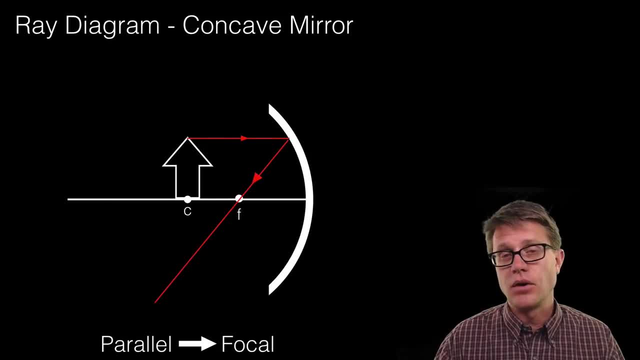 a parallel line, Then where does it go? Through the focal length focal point? Now I am going to start at the top, again through the focal, and then it is going to go parallel. And so where is my image going to be? It is going to be upside down, like that. Now you might. 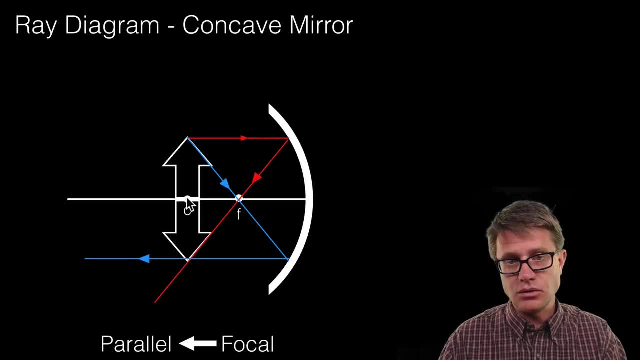 be thinking: how do I know where the bottom of it is? So imagine doing the same rules on the bottom. So on the bottom we could go parallel back through focal And then through focal back through parallel. So the bottom is going to be right where the top of that image actually. 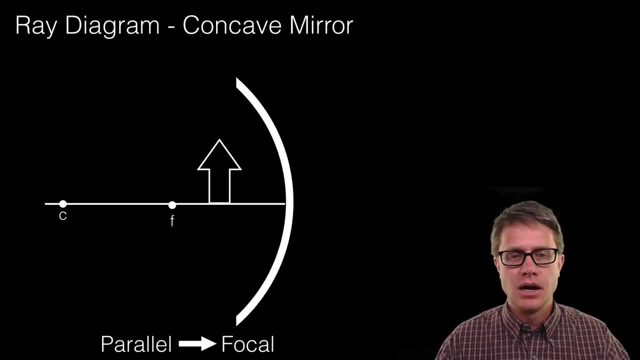 was. So you can see now it is the same size. It is inverted. Let's see what happens when you move inside the focal length. You can see that we have zoomed in here. That is where it gets a little bit crazy, And so this is the only different one that you really have. 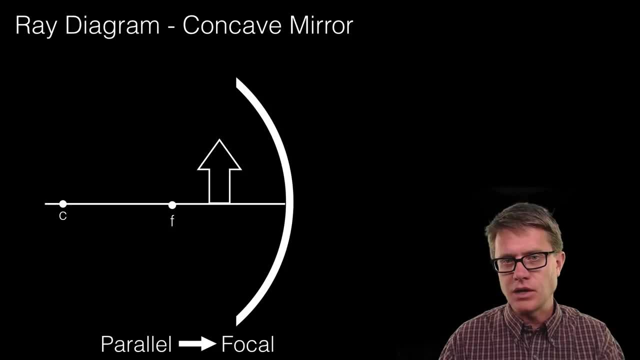 to draw. So let me draw it again. So I am always going to start at the top of the object. I go parallel to the mirror through the focal. So that seems easy. But now it is hard for me to go through the focal, And so what I have to do is actually turn it around and 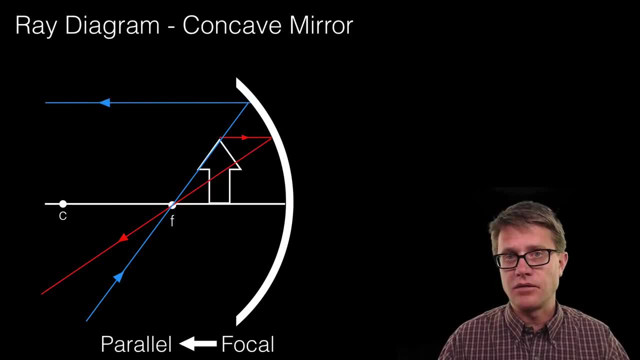 I would go through the focal like that And now I draw it coming off parallel. So it is a little bit different. But what is interesting, you will note, is that this ray and this ray, as they move away from the mirror, they are moving away from each other. They are not. 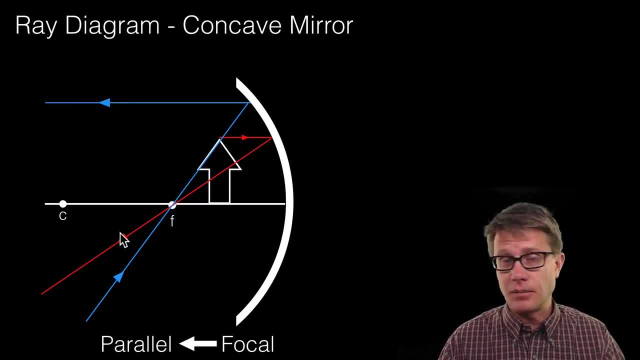 converging at any point They are diverging, And so that tells me that I am not going to find an image on this side of the mirror, And so what I can do is I can take those two rays and I can extend them into the virtual. 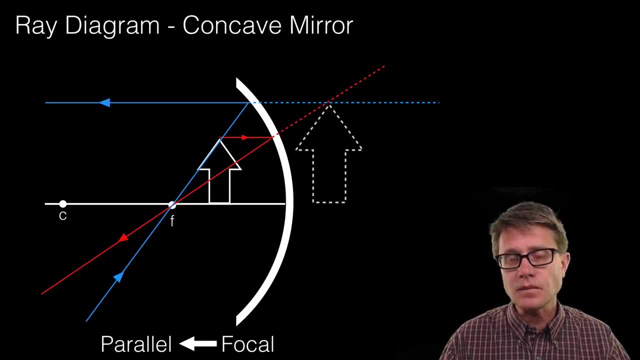 side of the mirror. And so where is the image going to be? It is actually going to be on that virtual size. It is going to be larger in size and it is going to be upright in nature. It seems a little bit crazy And remember, once we get into the focal length, then it 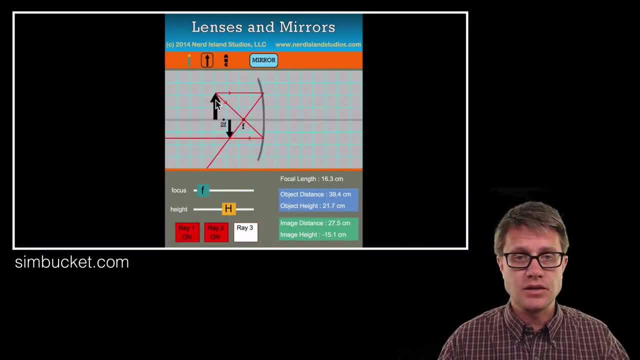 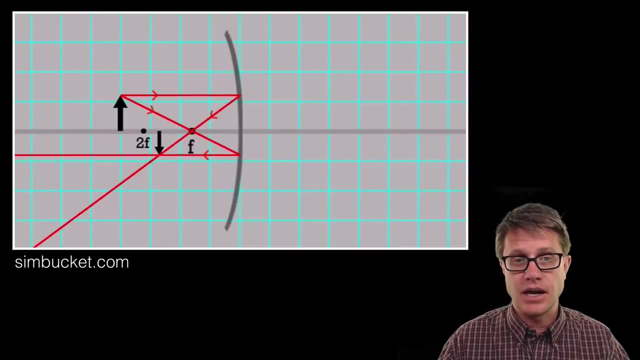 gets a little bit crazy. So let's make sure that this is true. So I have got a Simbucket simulation here. What you can do is you can move the object on the left side. You can see that as I move the object on the left side, we have got a real image that is inverted. 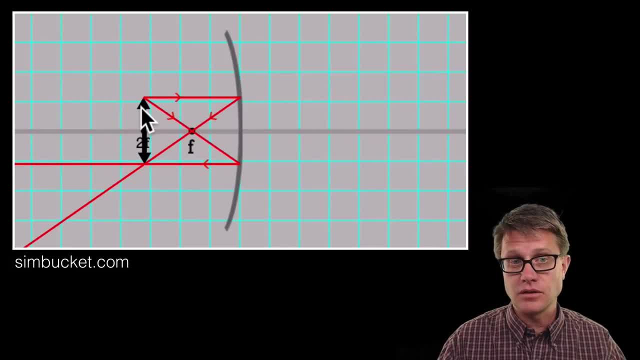 I made it a little bit smaller, so this works. Now we are at the center of our curvature. It is 2F, So it is upside down. But watch what happens as we approach the focal length. That image is getting bigger and bigger, and bigger and bigger Once we